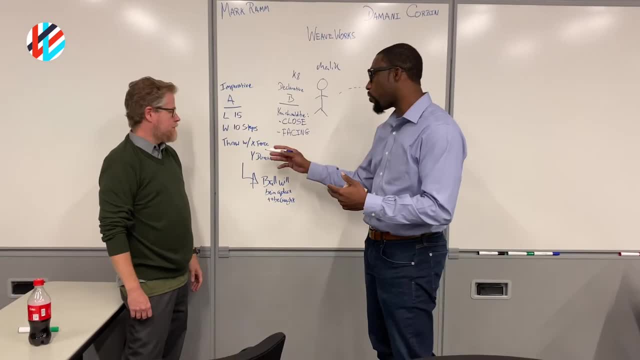 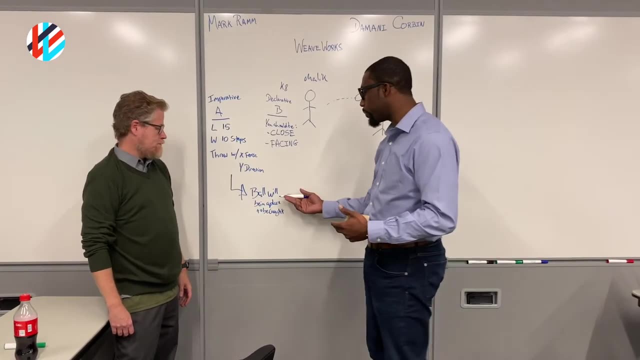 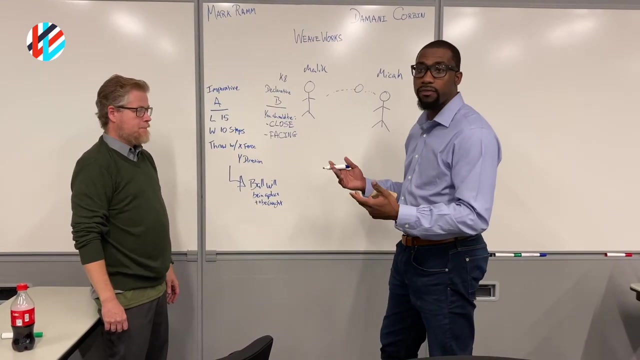 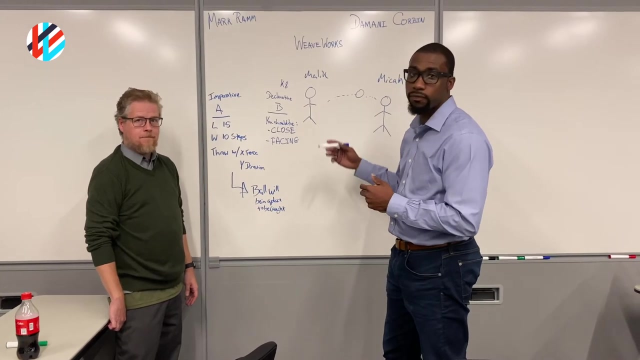 walk 10 steps to the right, then throw with X amount of force in Y direction And then that the end result will be: the ball will be placed, that his brother will be able to catch it. Another way of explaining to my child will be a declarative way and saying: Malik, you should be close enough, you should be facing your brother and you should throw it. 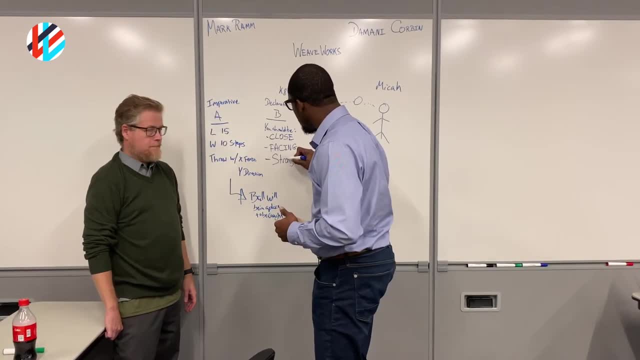 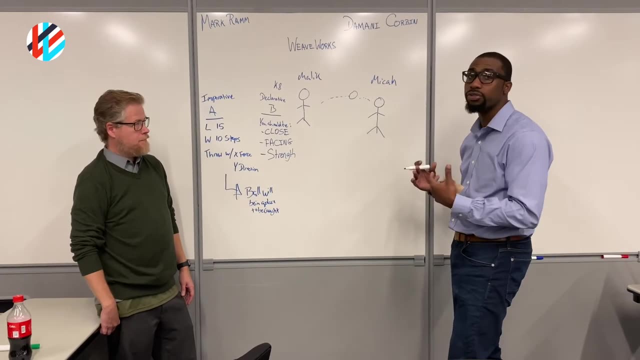 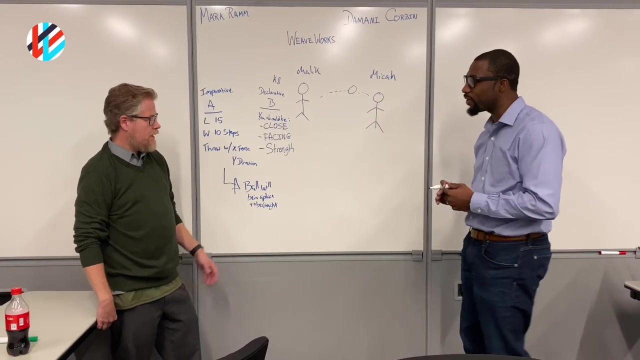 back to your younger brother, and I have not touched a ball out of there. That's what it will be for you Once you knowbilir that. leave it, You learn to get to your brother. So these are two separate or different ways of explaining to my children how to play catch. 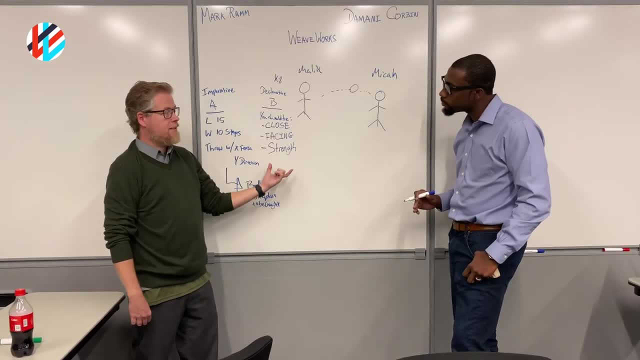 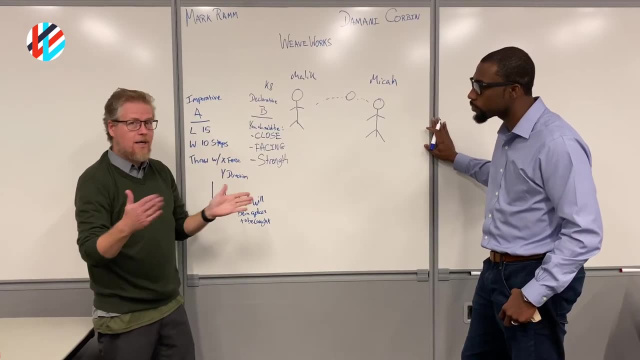 And I think that's a digestible example of what you're talking about and I will talk about it. And in the same way, Kubernetes says: this is the goal state. This is what I think you should, where we should end up adjust routines are we facing? How do I adjust routine? Am I throwing with enough? 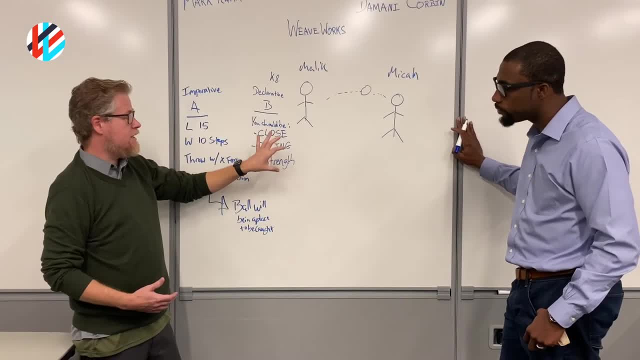 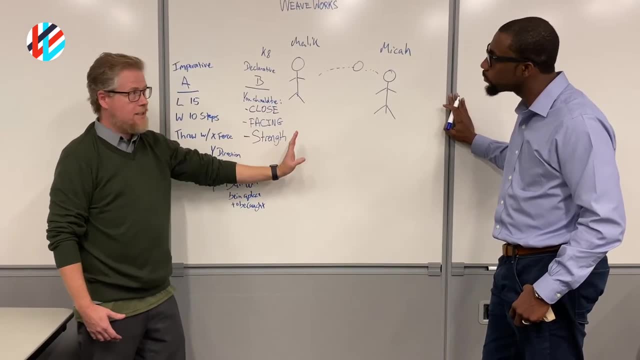 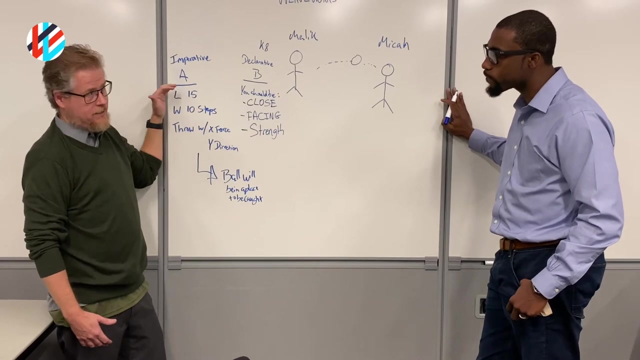 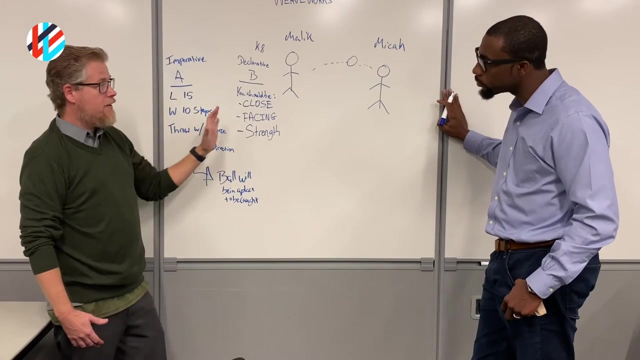 force. Kubernetes has a bunch of controllers that take a declarative view of what should be running and then make those into reality. The other approach is to try and do things one step at a time and get the same result. This is what you would do if you're just using bash to script, deploying those same services. The 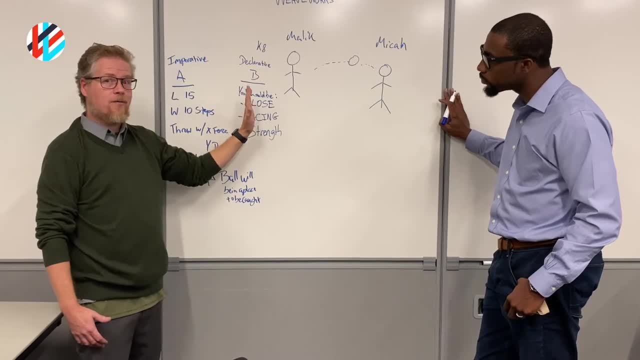 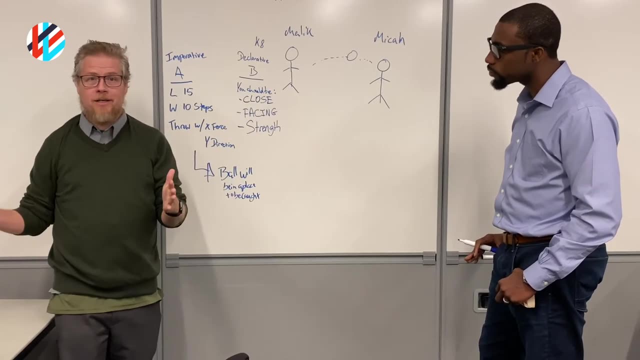 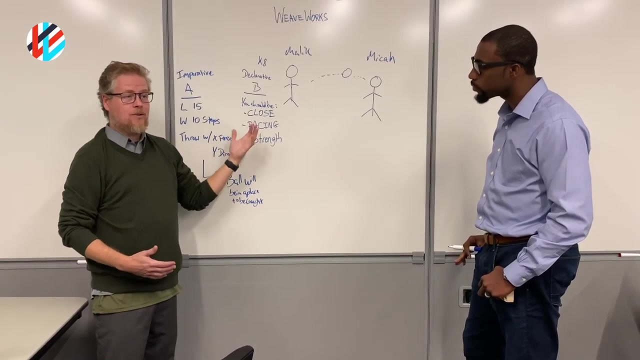 thing that is completely different here is that if there are failures, the goal state can say: oh, like your brother moved, you should turn because he's moved. Your brother is too far away, you should move closer to him. Those things can happen as real-time corrections, because what they are, what Malik has given, is a set. 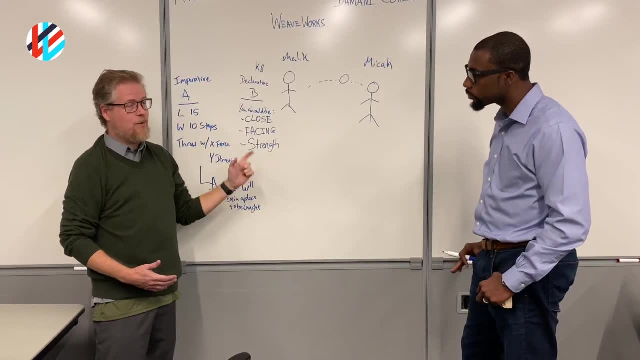 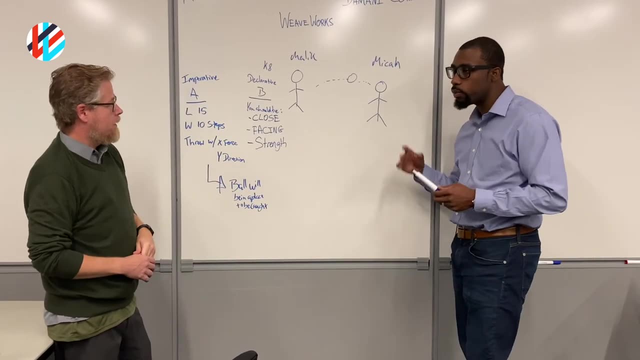 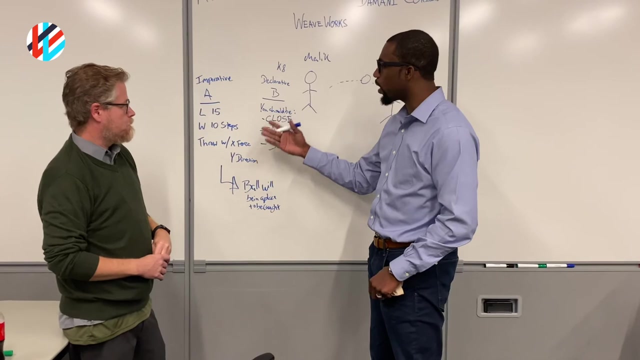 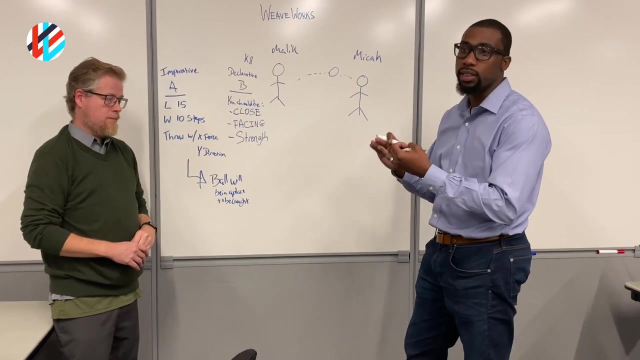 of goals for the system, How to do this, as opposed to set up specific instructions for what to do. Sure, so in Kubernetes, Kubernetes does a lot of magic and it automatically assumes it is smart enough to figure those things out, as opposed to other methods or other ways, in that it doesn't account for: is it raining, Is it windy, Is